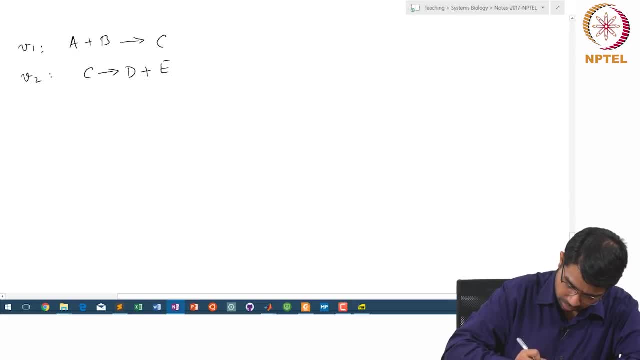 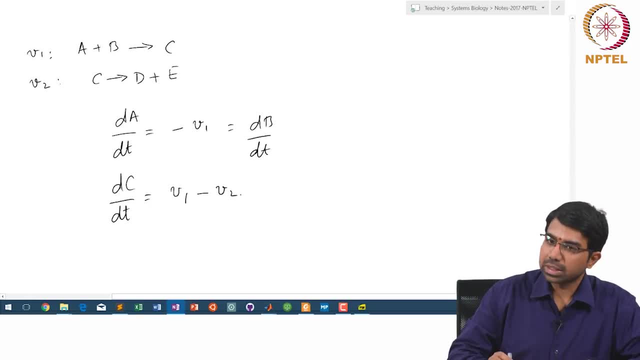 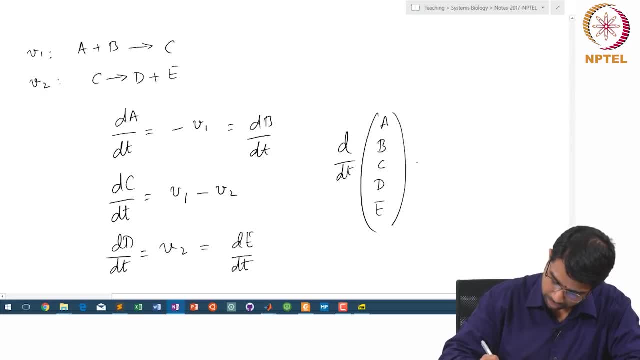 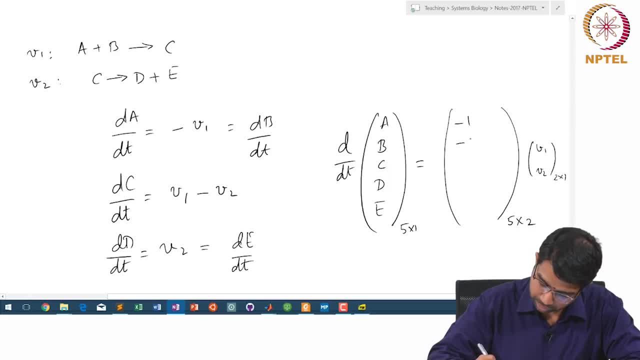 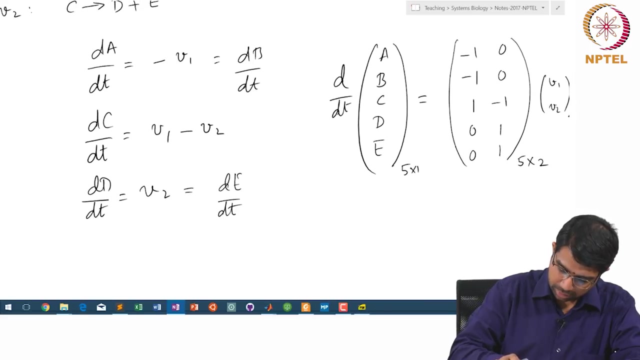 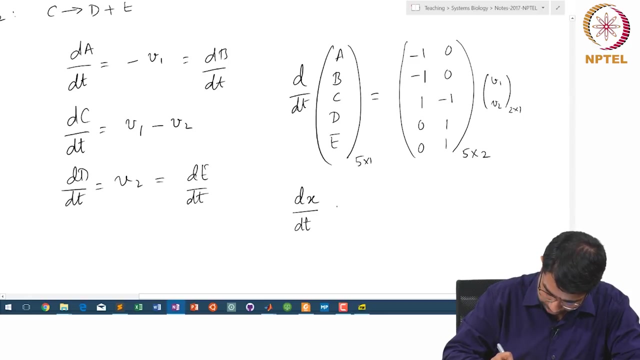 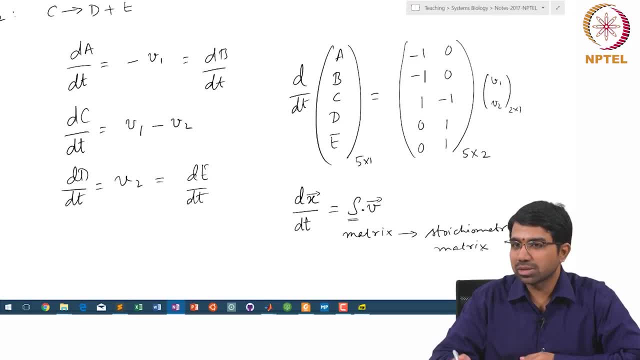 the next module of the course, when we talk about flux balance analysis and constraint based methods for studying metabolic networks. but this is very important to know right here. Why? Because these are your differential equations. If you are able to write expressions for all the Vs, you can simulate it. 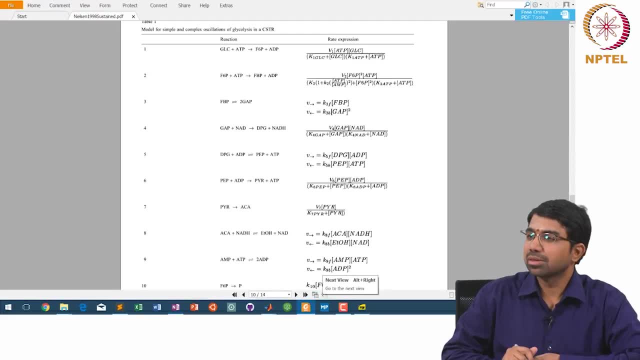 Let us go back. here are the expressions for all the Vs right. So your reactions are: GLC plus ATP giving F6P plus ADP. F6P plus ATP giving FBP plus ADP. Identify the coefficients for each of these. 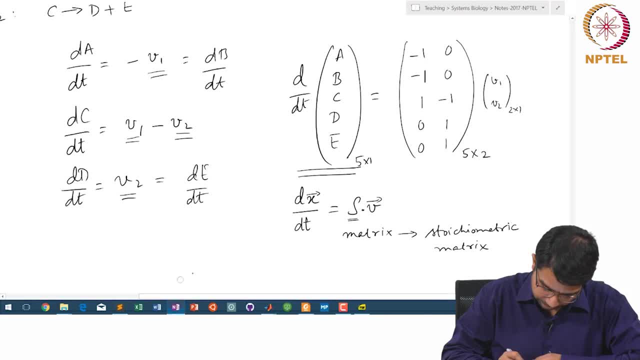 If you look at this a little more closely, what are these coefficients In this matrix? The stoichiometric coefficient? negative for reactants, positive for products. that is it, So you do not have to actually worry about writing these equations out. 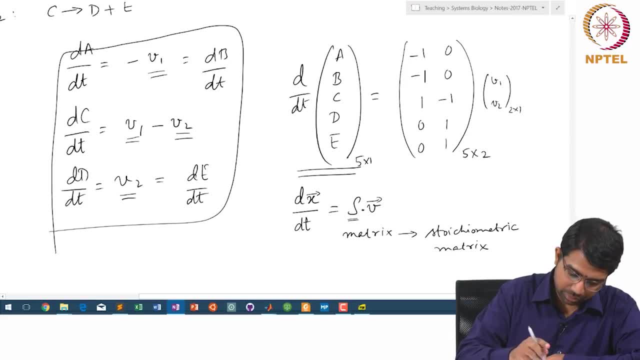 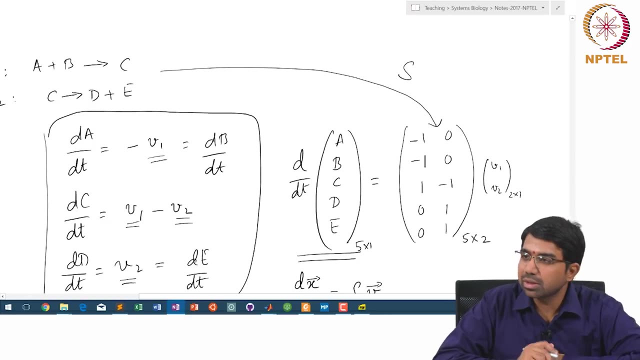 You really do not have to worry about writing out all these equations, right? So you can. basically, the moment I give you a list of reactions, you can directly write out the stoichiometric matrix, which is what you can do in this example. potentially, 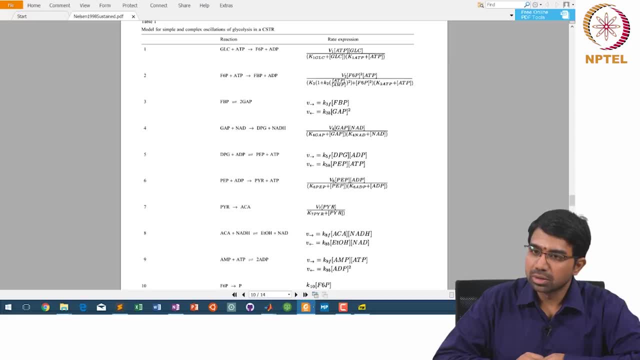 But writing it in one sentence is not enough, Right, Writing it in one sentence is not enough. While coding it, we have to hand-code everything. We will have to hand-code everything. So, thankfully, somebody has already done this. So, if you look at, 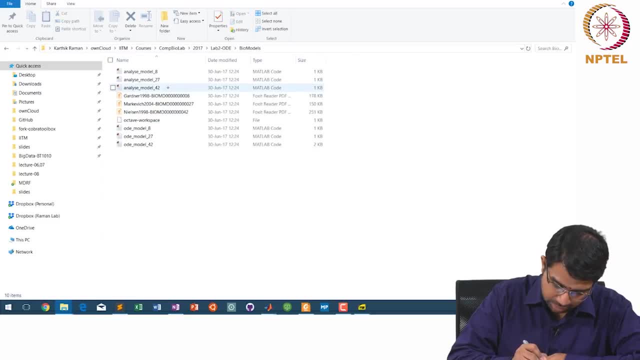 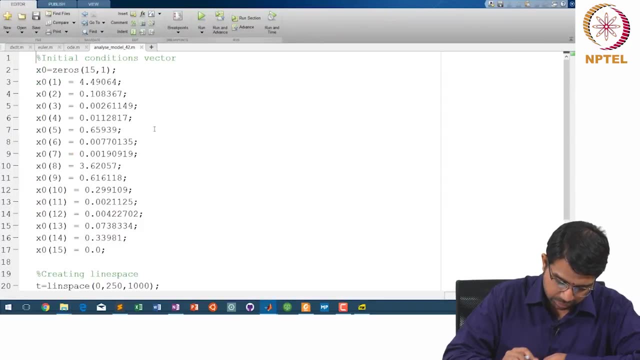 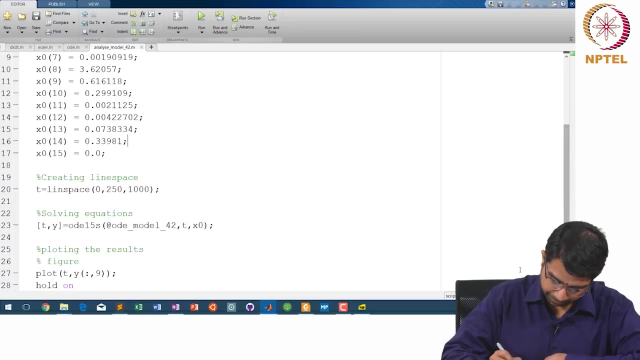 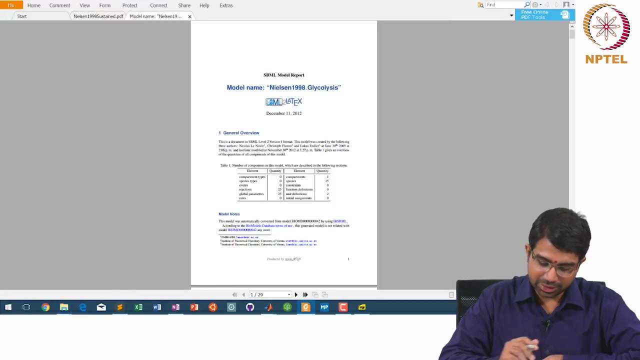 So this kind of a file is available for you to use. I am going to show you how to use it, Okay, Okay, Okay, Okay. So this is a file from biomodelsnet And in fact, this is a very interesting file. 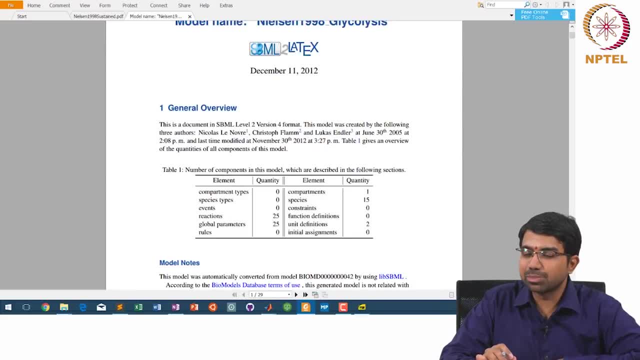 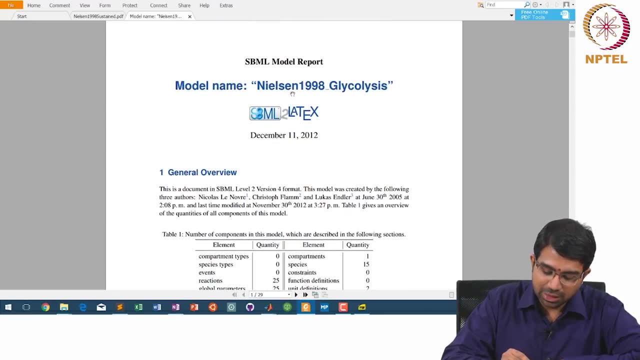 So biomodels also allows you to get an SBML report, a PDF report of any SBML file. It has curated several SBML files So it calls this file Nielsen 1998, glycolysis, And this has a lot of details. 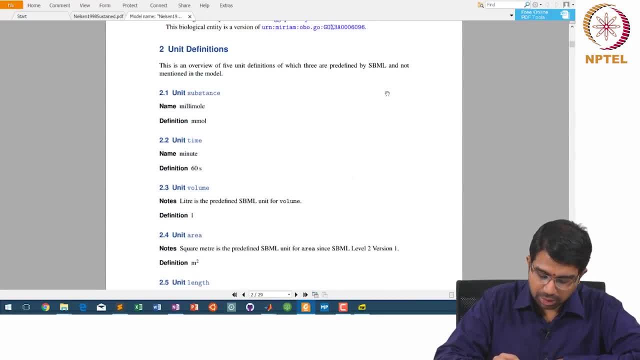 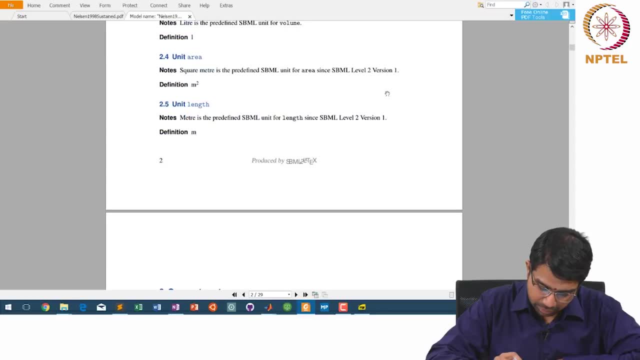 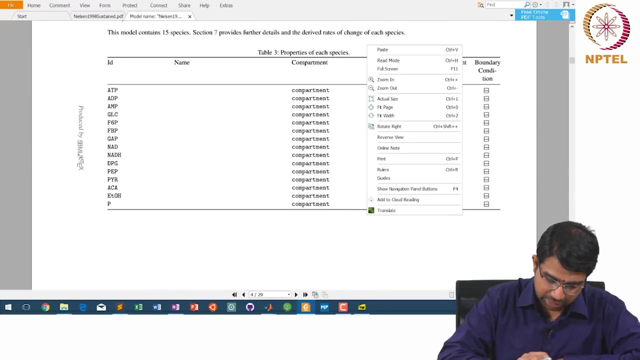 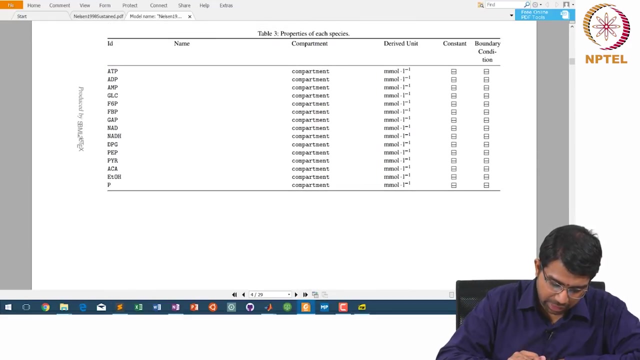 Okay, Okay, Okay Okay. This is essentially from the SBML, Right, If you remember SBML from a few classes ago. So the compartment, let us just cut to the chase. These are your species. So you want to do a DAT by DT, DADP by DT, DAMP by DT, all of these. 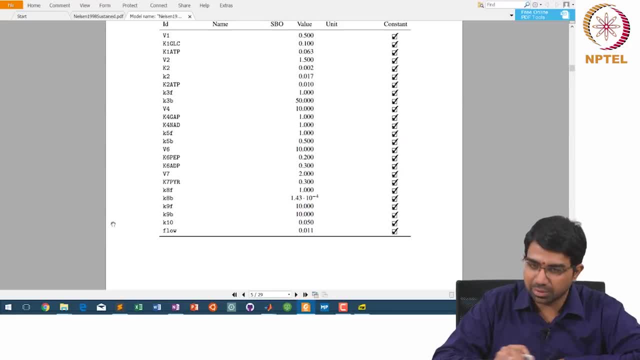 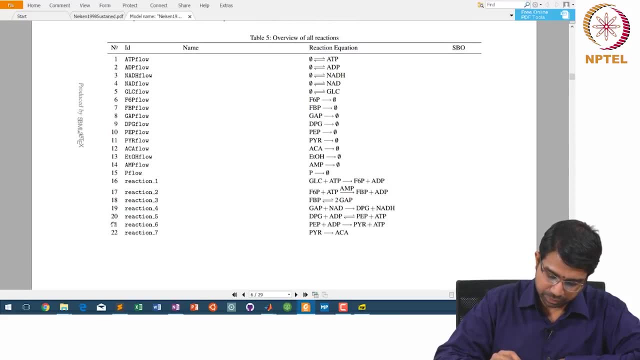 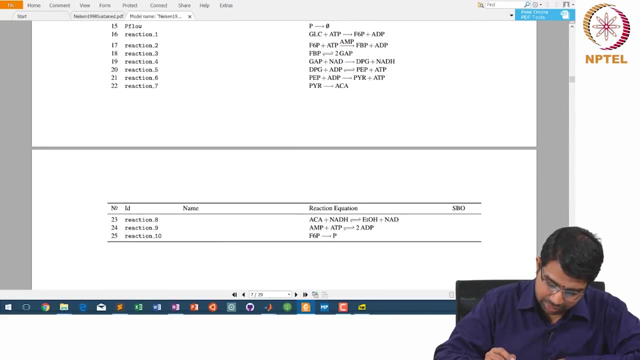 Okay, Okay, So these are parameters. They are in the manuscript which I was just showing you And these are all your reactions. These are ATP input source and sink reactions, but these are your main reactions. It you have about 10 reactions. 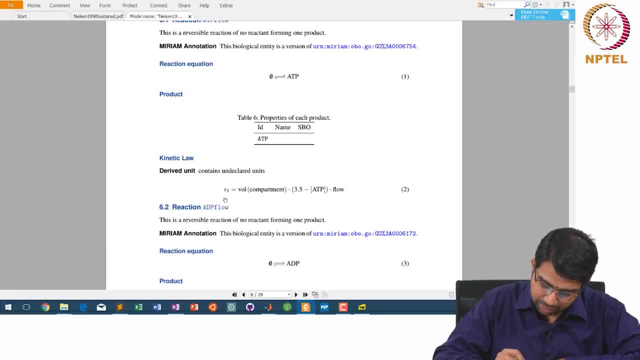 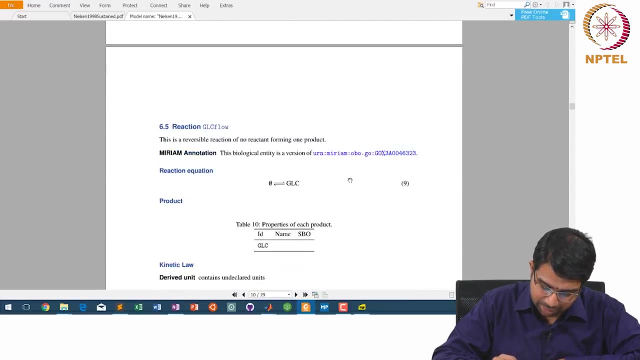 And the good point, good part- is it already gives you V1 equals volume of compartment. You can keep that as 1 if you want. V2 is 3.5 minus ATP into flow. Let us look at. so this is our ATP flow. let us look at the other reactions. 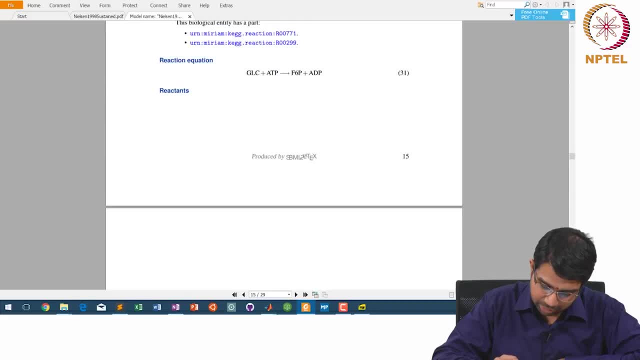 These are. this is essentially a stoichiometric matrix derived from the stoichiometric matrix. So V16 is this, Reaction 2 is this, Which is this. You need to write those out. let us skip to the metabolites. very nice, DATP by DT is: 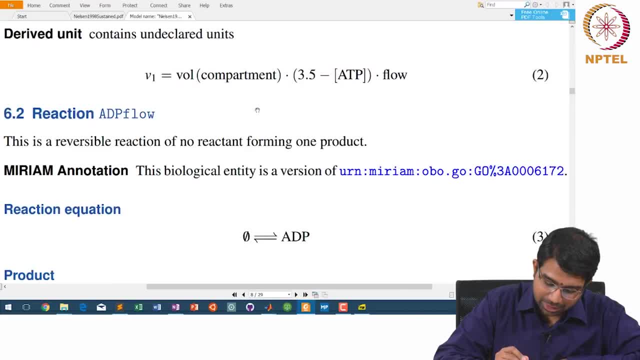 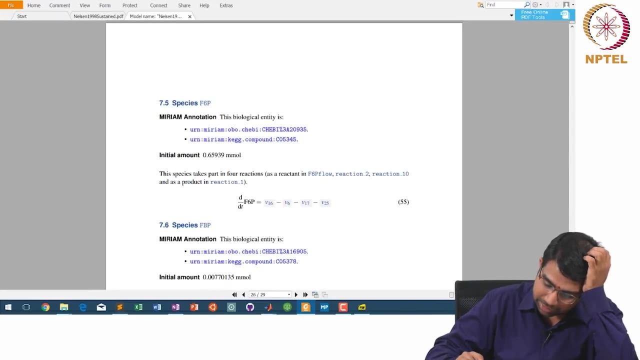 V1, it is also hyperlinked by the way. you can just click it and go to V1, right? So DNAD by DT is V4 plus V23 minus V19, DF6P by DT is V16 minus V6 minus V17 minus 25, and. 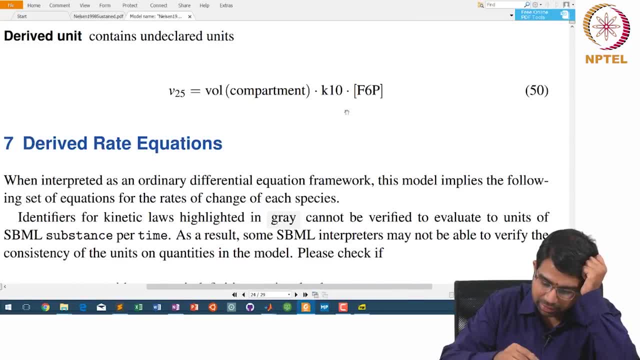 so on, and all these have been defined previously. what is V25?? It is here. So biomodel actually gives you files for Octave, not for MATLAB. you can just make a few small tweaks and use it with MATLAB. there are also other tools that you can use it with. 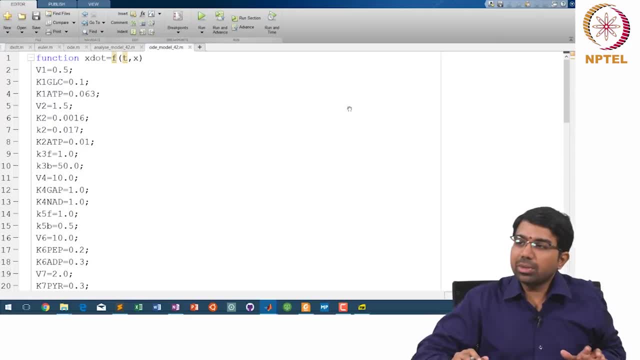 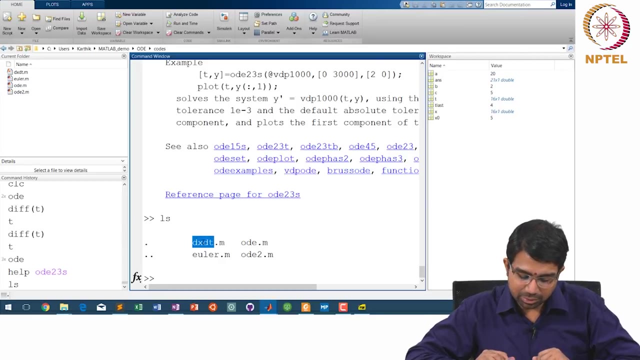 So how does this look? I would recommend this architecture for any ODE solving problem. you first set up a file, just like we had in the previous example, ODEM, or rather analyse the ODE and your DXP by DT, which is basically something like: you know, the ODE of the model, model ODEM, right? 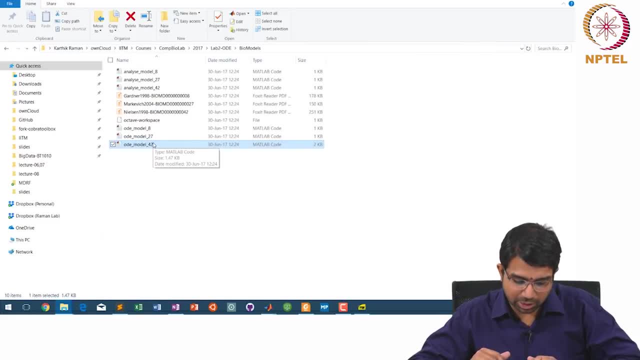 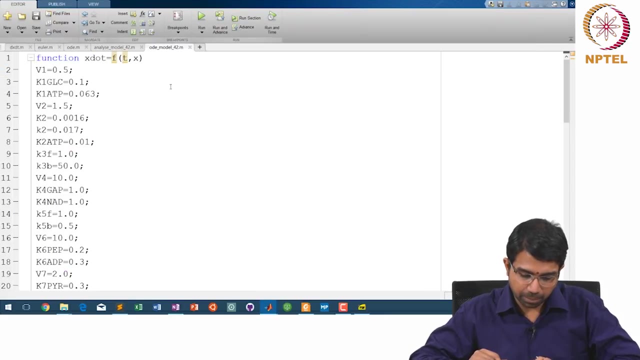 So I have something like that here. so I have ODE model underscore 42.M and analyse model underscore 42.M. 42 happens to be the biomodel's ID for this particular Nielsen glycolysis model. Student is answering the question. 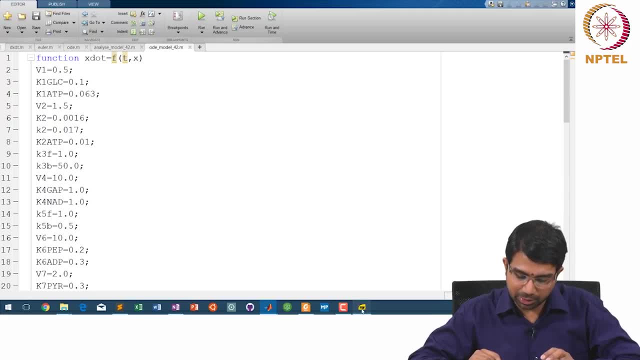 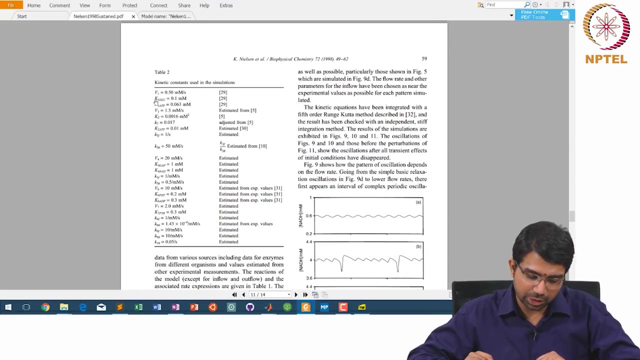 And then you code all these parameters. Okay, All these parameters are available in the manuscript. if you look at it carefully, The next page, right. So it says V1 is 0.5, K1-GLC is 0.1 millimolar, K10 is 0.05 per second, and so on and so forth. 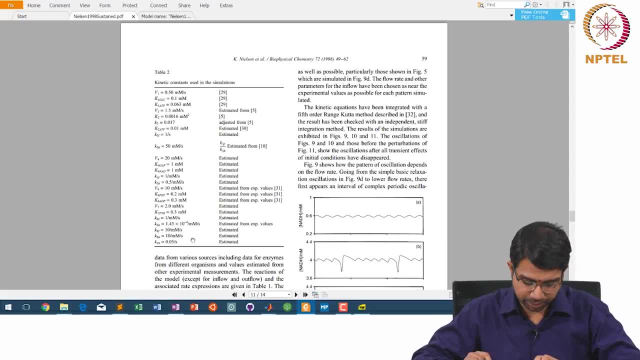 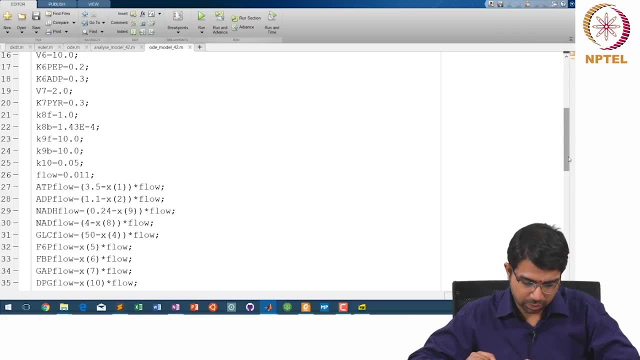 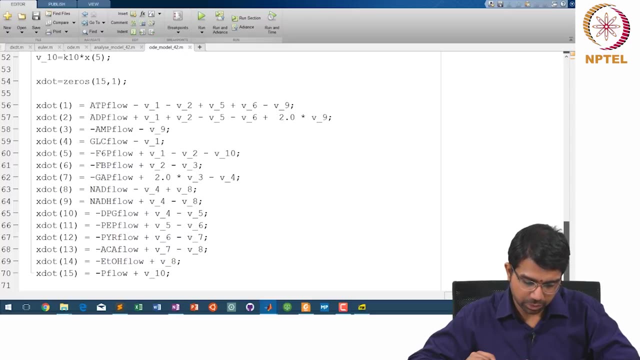 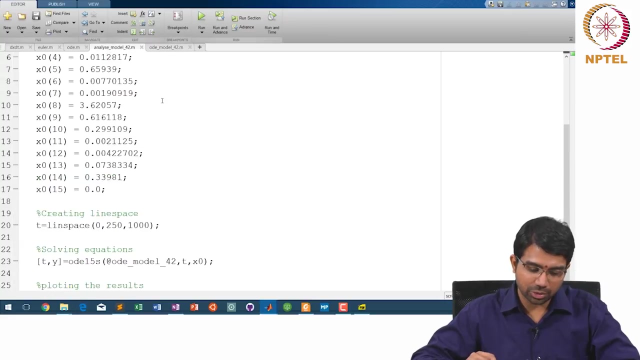 You have all these values that are listed here, and so it goes. You have all the equations listed here: X dot 1. is this? X dot 2? is this X dot 15? is this? Now you can actually solve this. You can use analyse model 42.M to solve it. 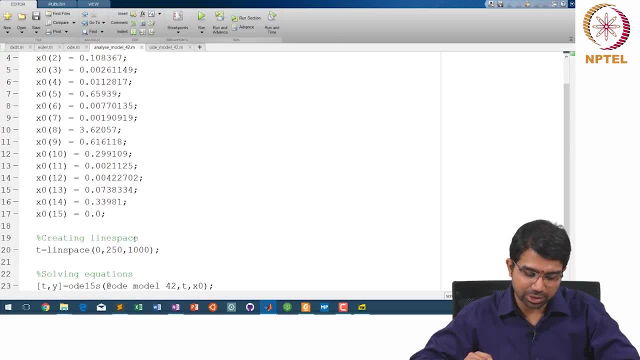 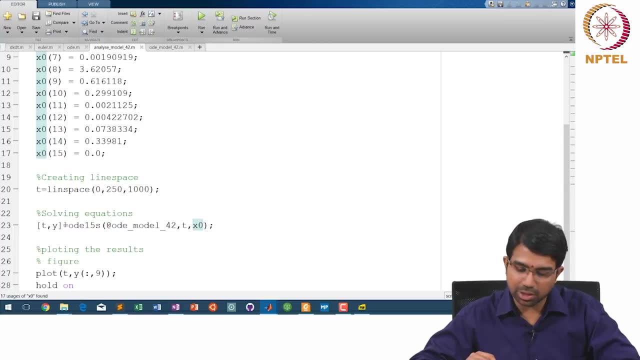 What do you need to do here First is set up the initial conditions, Okay, Then create a vector where you want to simulate it. Then basically the same old thing: T, Y is ODE, 15S of ODE model 42, T Y0, Y or X, yeah, 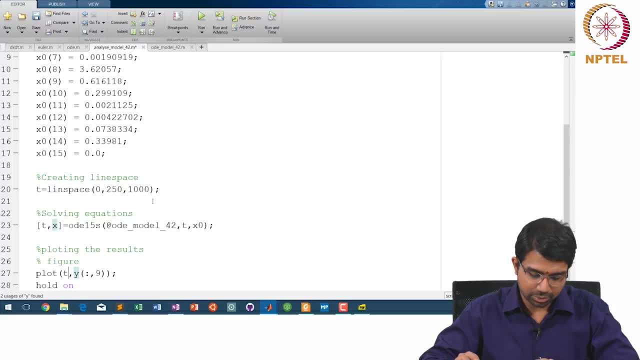 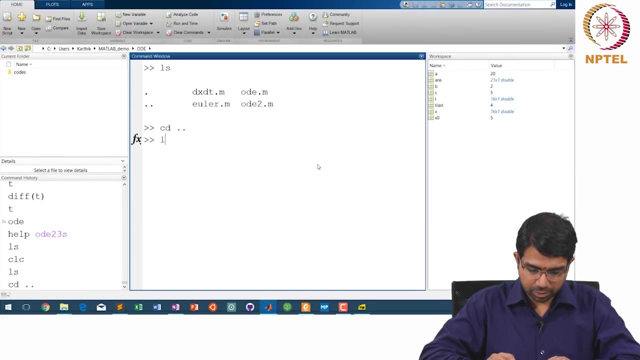 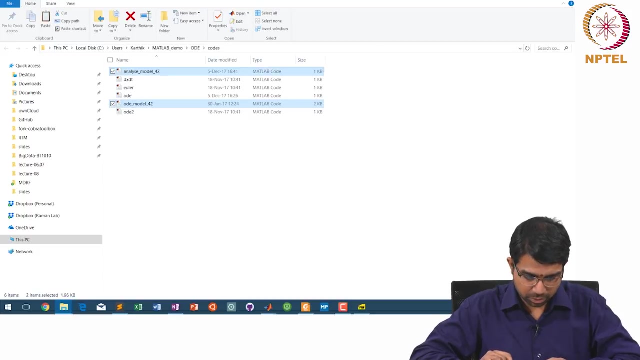 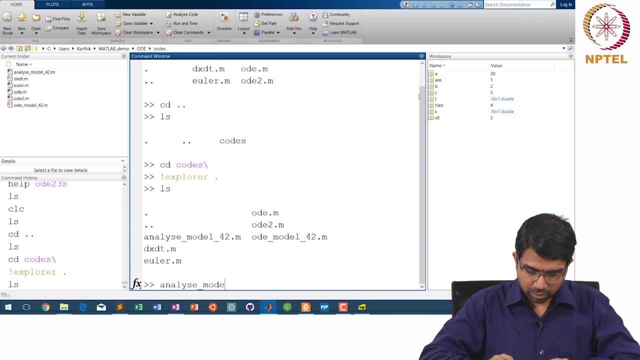 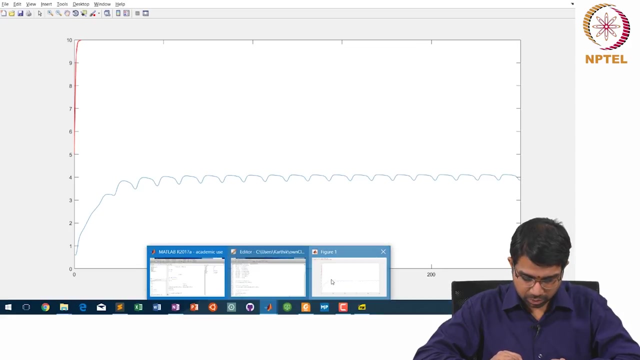 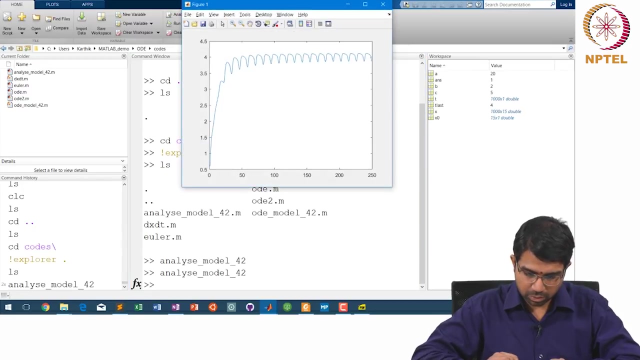 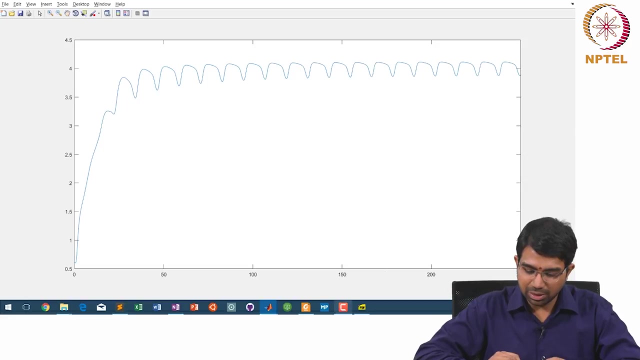 You can probably have it as X here, Okay, So let us just run this. Okay, Okay, Let us run this. You see, much like the same oscillation that is there in the paper right, something of. 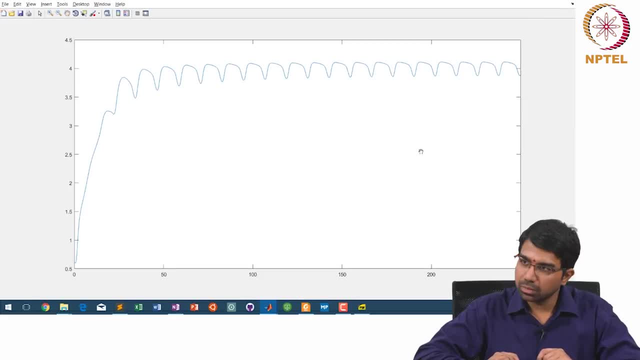 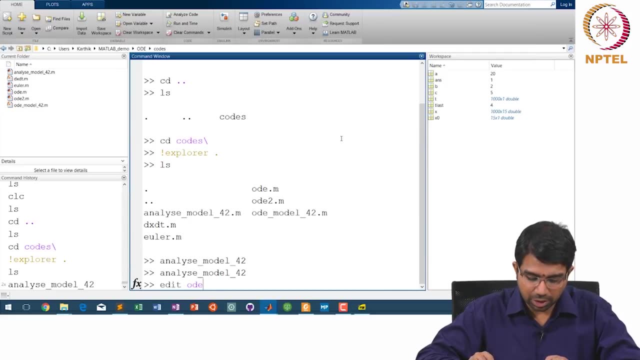 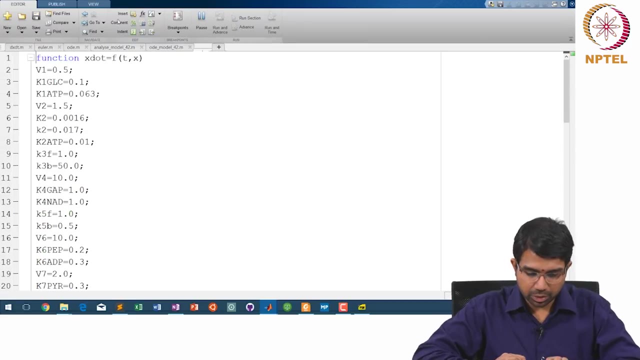 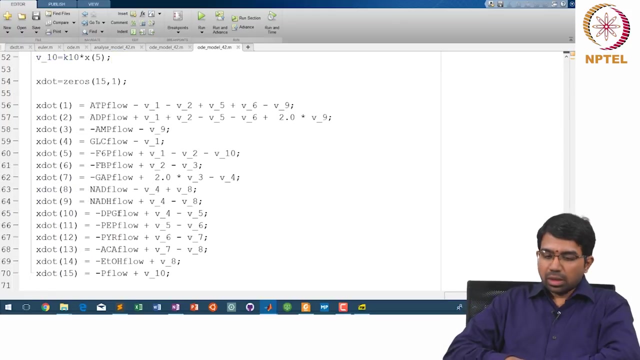 this sort the equations. can we look at the mat equations? so basically call them as: x? dot is f of t x. essentially you can get it from the stoichiometric matrix. So this is a vector Having x1 dot, x2 dot, x3 dot, all your species. 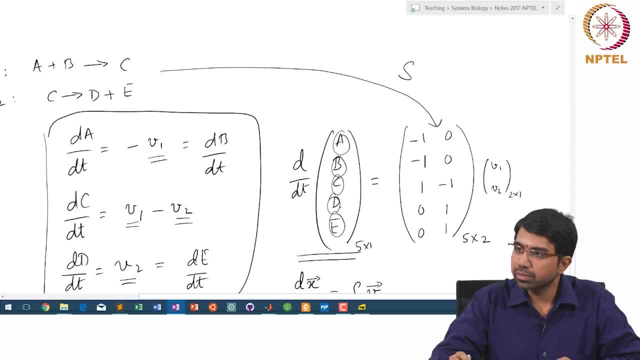 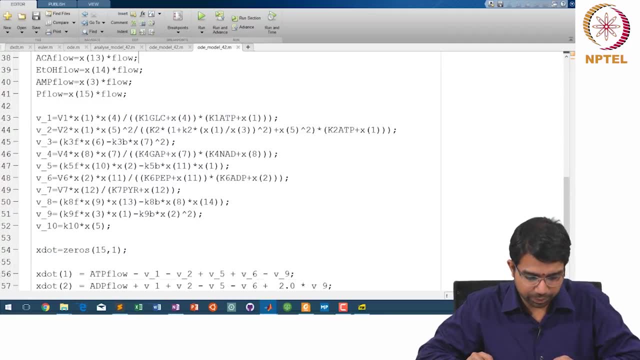 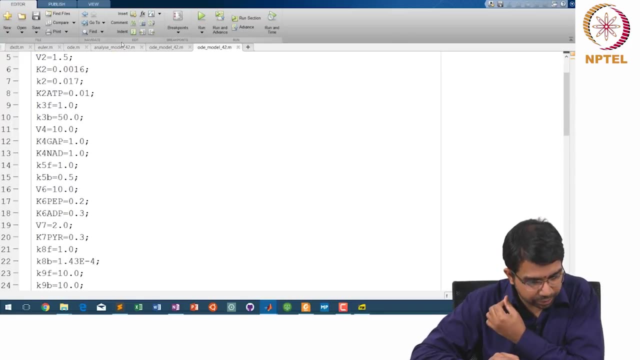 So we have 5, okay, so we need 5 initial conditions, Not 5, so here there are many more metabolites. there are 15 metabolites. You have 15 initial conditions. if you look up, The initial conditions will be set up here. 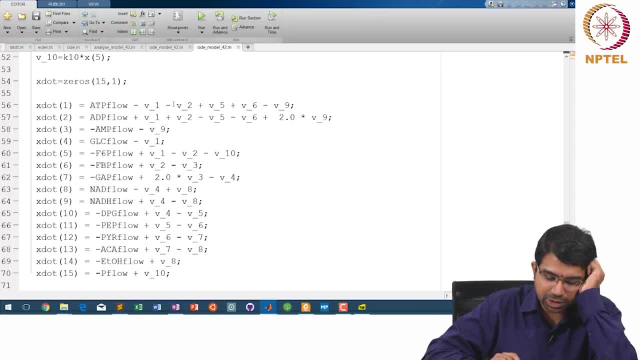 X1 is ATP, x2 is ADP, x3 is AMP, GLC, F6P, BB, Okay, Okay, FBP, so on ETOH, right? so all your glycolysis parameters and phosphate, whatever, all the. 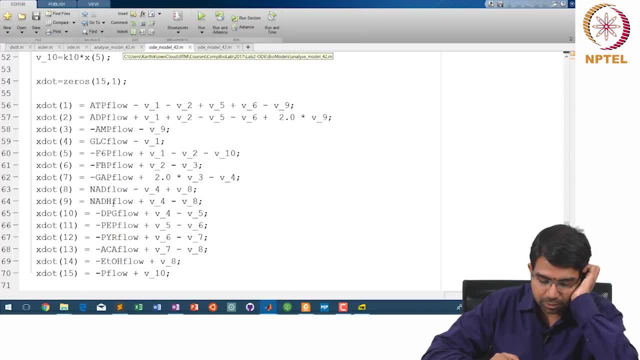 metabolites involved in glycolysis: bisphosphoglycerate, phosphoenolpyruvate, pyruvate acetate, ethanol, misaldehyde, phosphate. So you can see that ATP is present in B1, reaction 1, reaction 2, reaction 3, reaction. 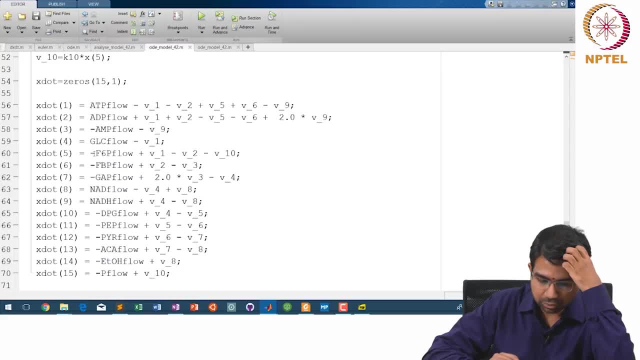 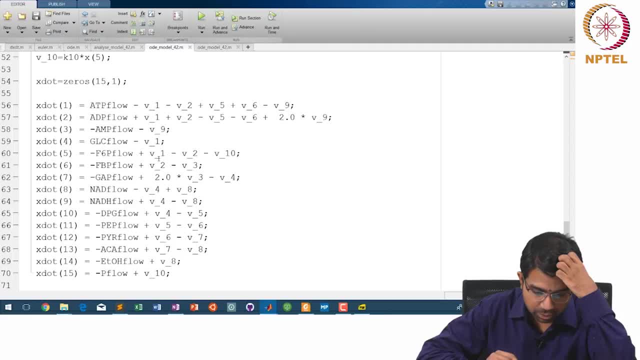 1. 1. 1. 1. 1. 1.. Then what is ATP? ATP flows, That is like an input sort of to the whole system. Yeah, because if you need a steady state of glycolysis, you need a steady supply of ATP. 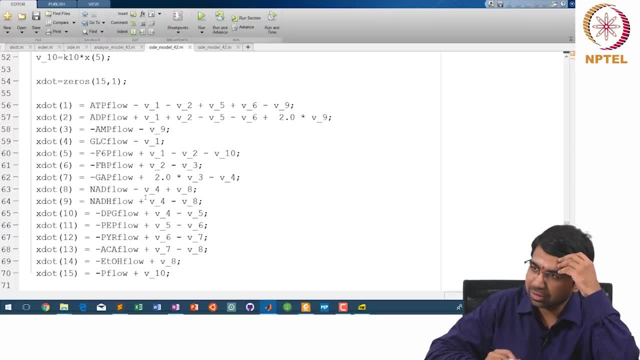 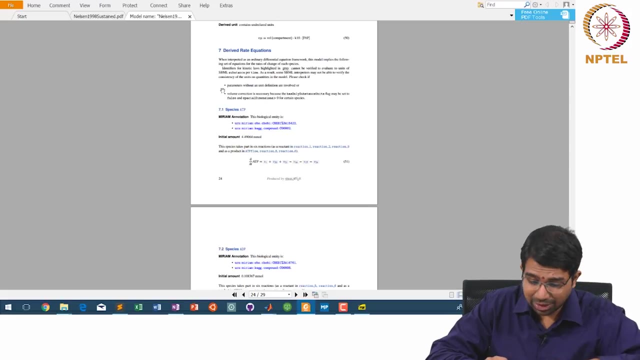 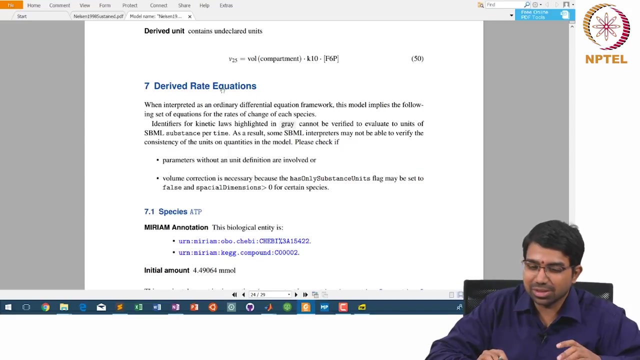 right, Okay, All of these actually in steady state. This model is described in great detail in this paper and also all the mathematical details are basically in fact. this is very interesting. all this information is encoded inside your SBML file. This is just literally an SBML to PDF kind of routine that was run to extract all this. 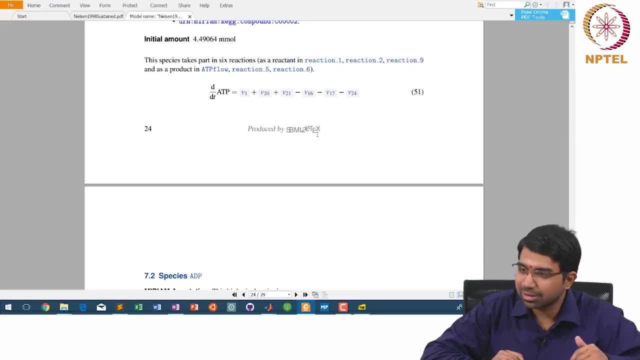 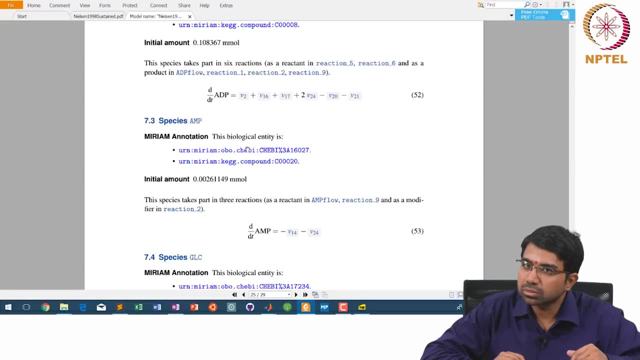 information out. So it is actually done by SBML to LaTeX. So x dot should contain variable in terms of that x1, x dot of 1 should be in terms of x1.. No, Not necessarily If it is. 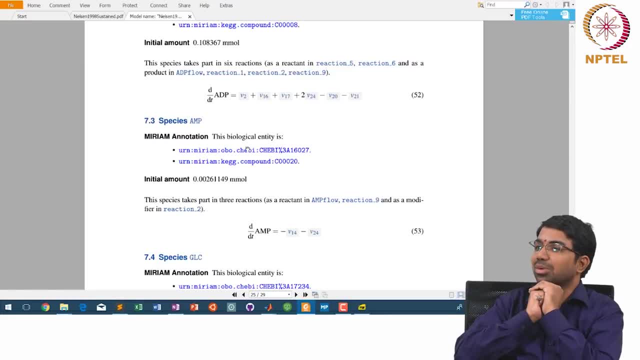 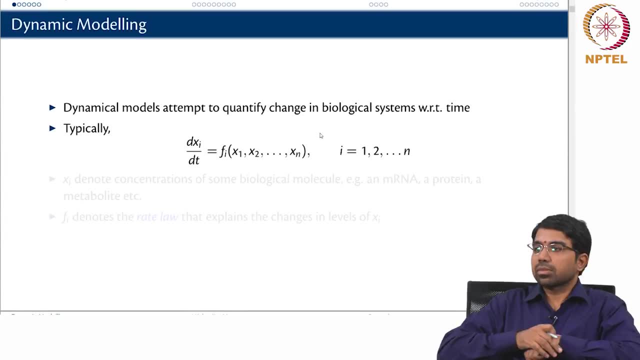 It is multidimensional right. So no problem, See, if you remember the very first slide for today, dxi by dt is fi by dt. Fi of x1 to n does not matter. So you will have to figure this out, right. 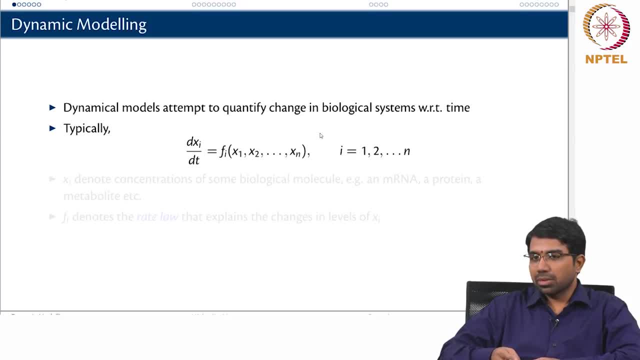 You have to try out a few examples. It is not difficult but it involves rigor. You have to be very careful. You cannot make, like some minus 1, plus 2 mistakes kind of thing. You have to rigorously set up the equations. then you can simulate them nicely. 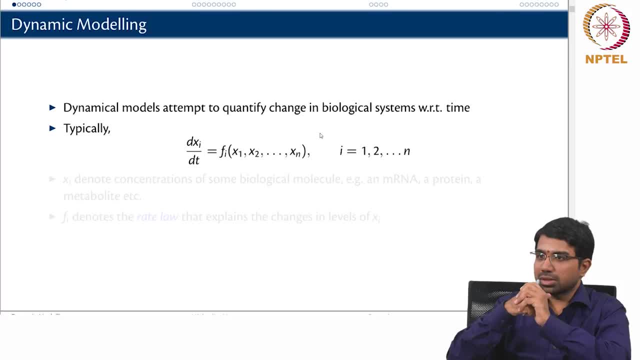 I will share these files with you. It will become clearer. You need to take a look at this file again, This analyze model, ODE model. all of these files I will share with you. Good, Any questions, Sir, there is actually an ODE package in Octave, correct?